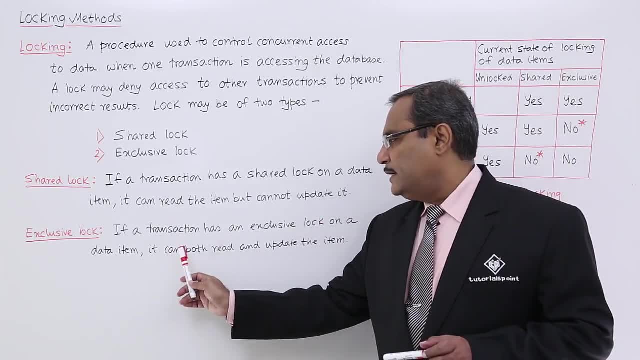 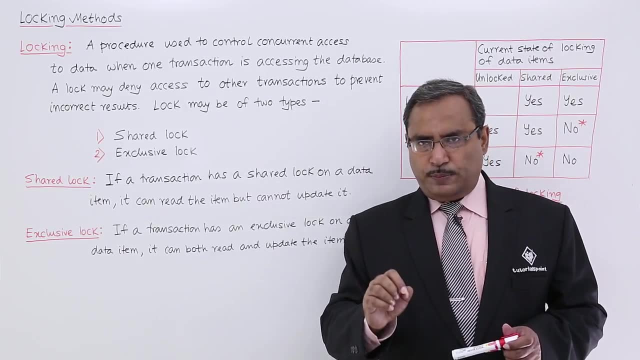 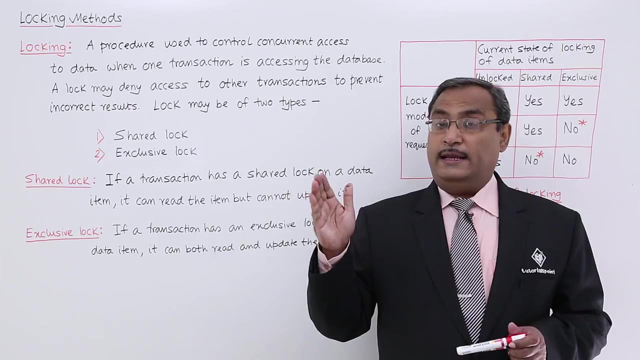 transaction has an exclusive lock on a data item, it can both read and update the data item. That means when a transaction will have the exclusive lock on a data item, then the transaction can perform both read and write on the data item And if other transactions will come to do the exclusive lock of 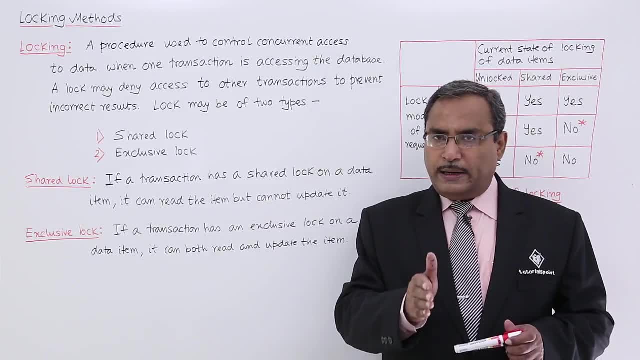 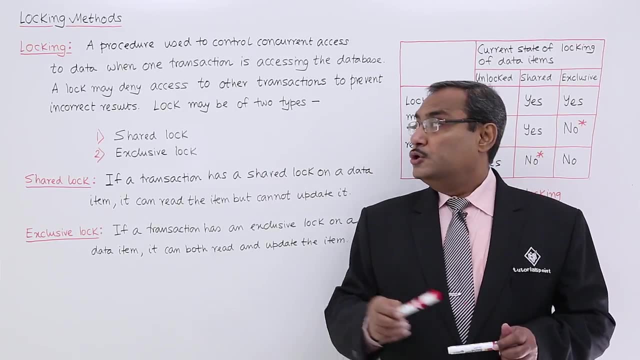 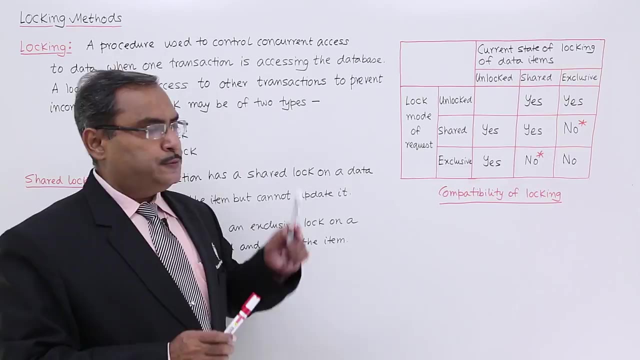 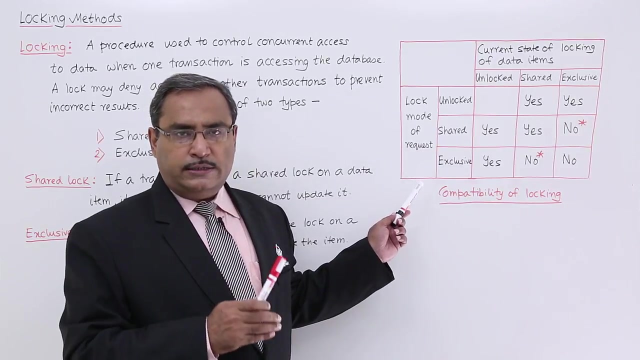 the data item, as the data item has already been locked by the prior transaction, so they will get a share lock. So this is the definition of locking and types of locking. So now let us go for this respective table. and it is compatibility of locking. Lock mode of request: One transaction has 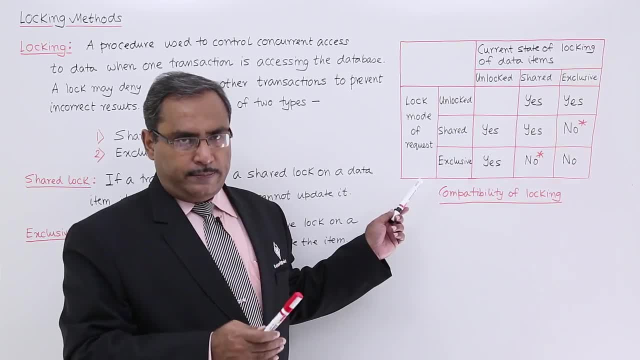 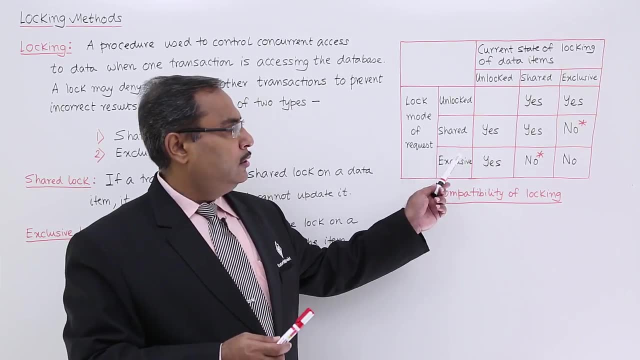 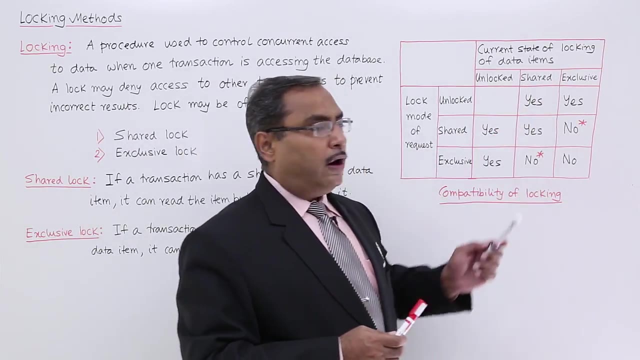 requested some lock modes on a data item, So let us suppose it is unlocked. The request is unlocked, or request is to get a shared lock. Request is it to get an exclusive lock, So let us suppose it is an exclusive lock on a data item. Current state of locking of data items. Initially, the data item is: 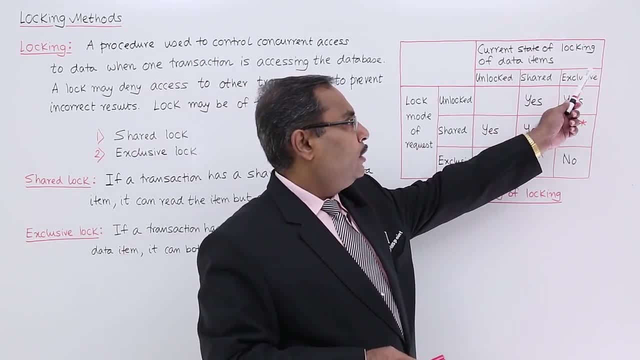 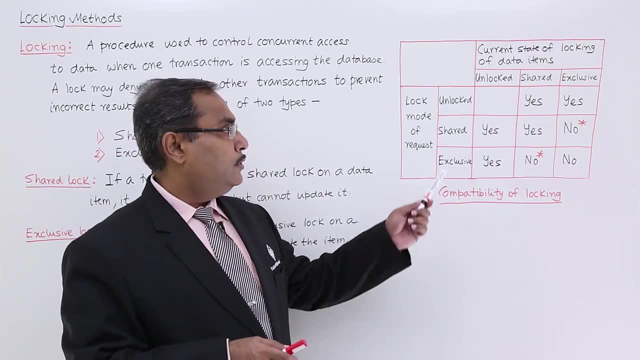 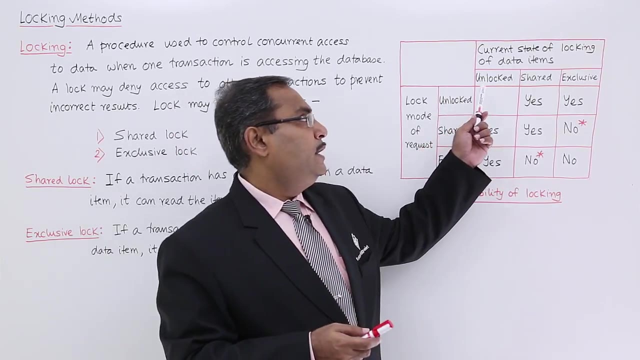 in the unlocked state or in the shared lock state, or it may be in the exclusive lock state. So let me let me go for that which is applicable and which is not applicable. So if a transaction goes for unlocked request- unlocked state request- of a data item, then if initially the data item is 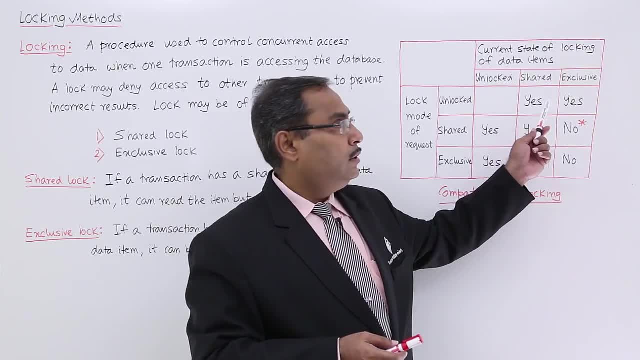 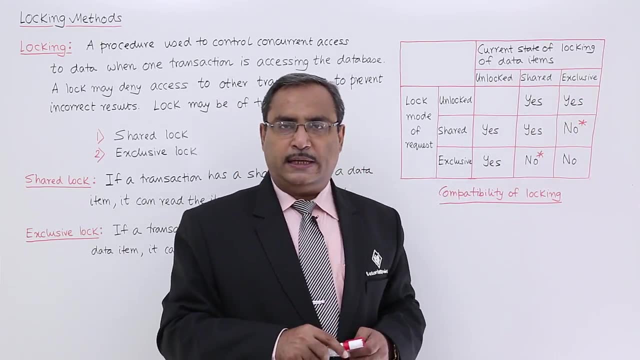 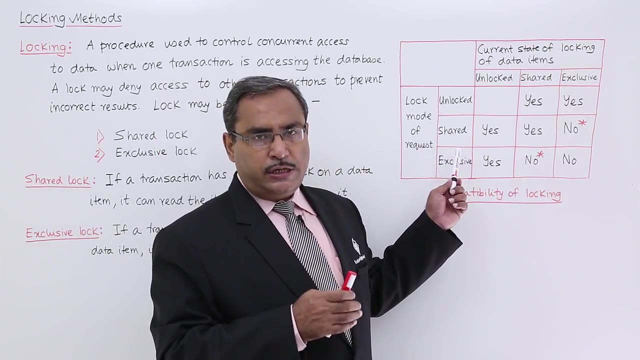 locked. if the data item is initially shared lock, then it can be unlocked. The if the data item is initially exclusive in the exclusive lock, then data item can be unlocked by the respective transaction who had that exclusive lock on the data item. If a transaction is having a shared 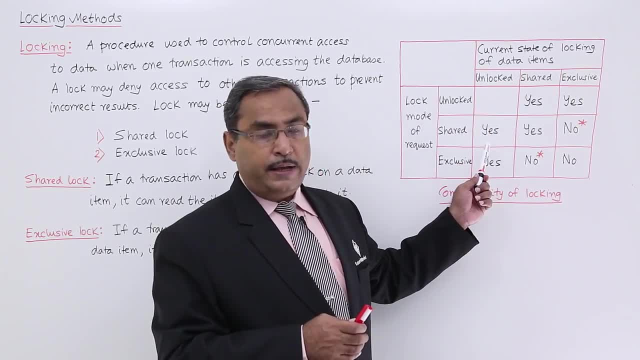 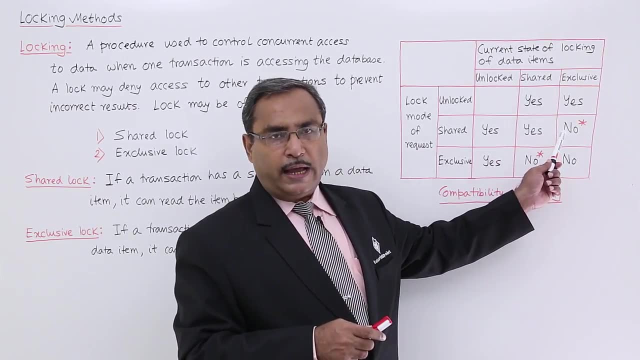 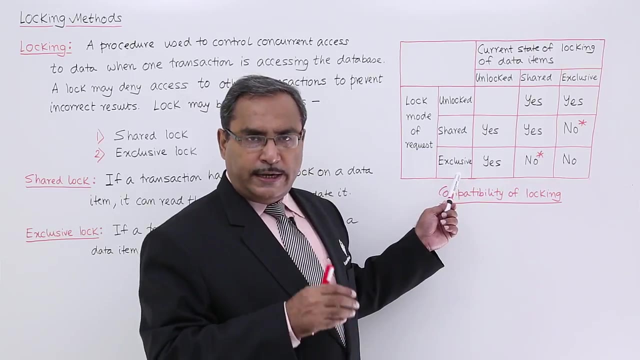 lock. in that case the corresponding data item can be unlocked, can be requested for shared lock by the other transactions and exclusive lock is not allowed in that case. That means from shared lock to the exclusive lock. not allowed In case of exclusive lock if the data item is. 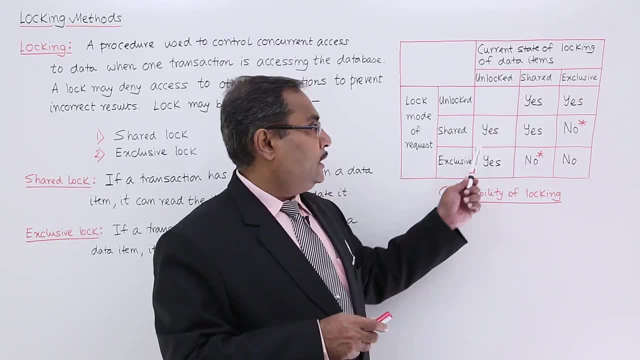 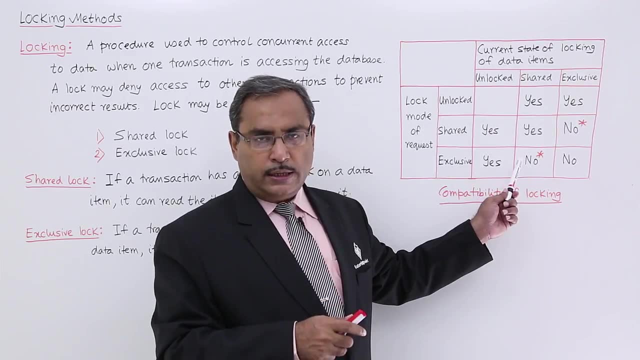 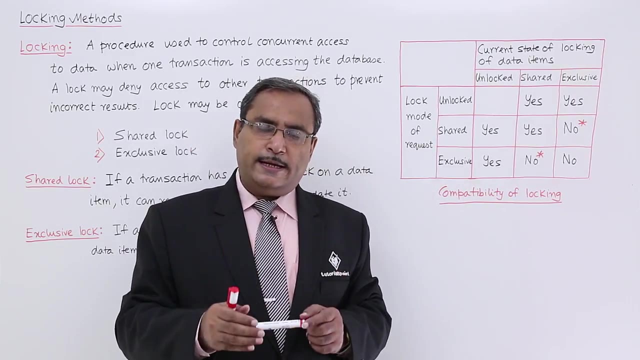 already under the exclusive lock of a transaction, then unlocked request can be granted. Shared lock request cannot be granted because it is already in the exclusive lock, but exclusive lock request will be also will not be granted. That means already the data item has been under the exclusive.